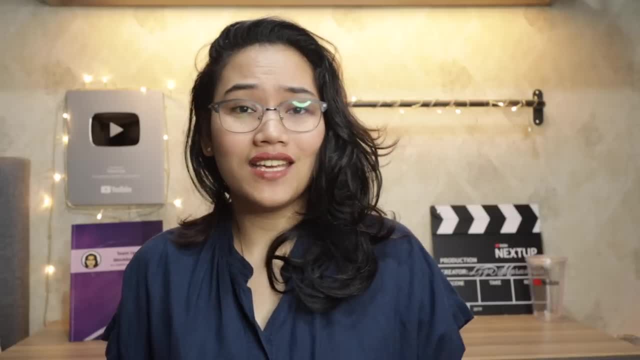 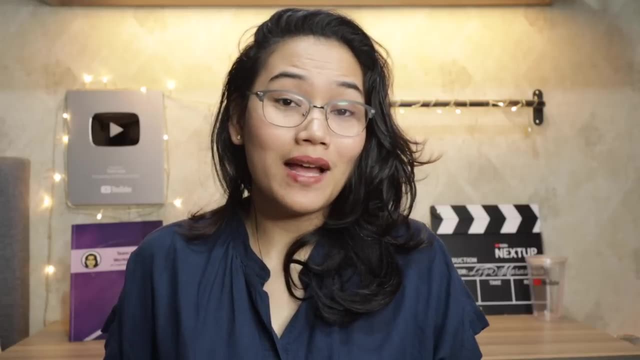 prime number. What's the next composite number in the series? Whatever that is, And it's good if you have these fundamentals. That's why I'm holding this. Hopefully I'll post this before your next exam so you can use it. And just a quick little plug if you're interested in the reviewers that: 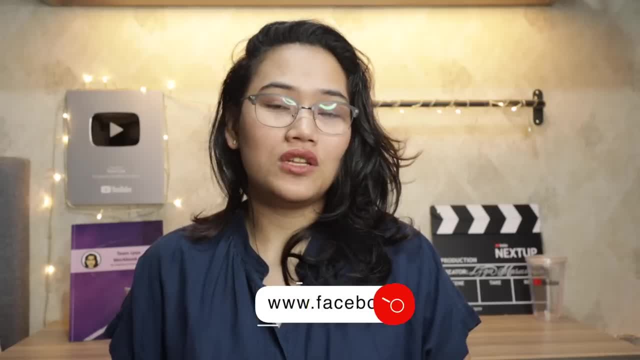 I made. if you want to join the online or live review events, you can go to wwwfacebookcom- slash Team Laika for more information. And now that I have that, I don't know if you're watching this live or not, but, by the way, I'm going to jump into my discussion. I'm going to 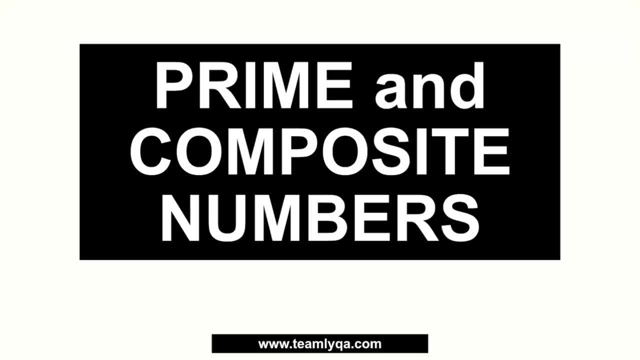 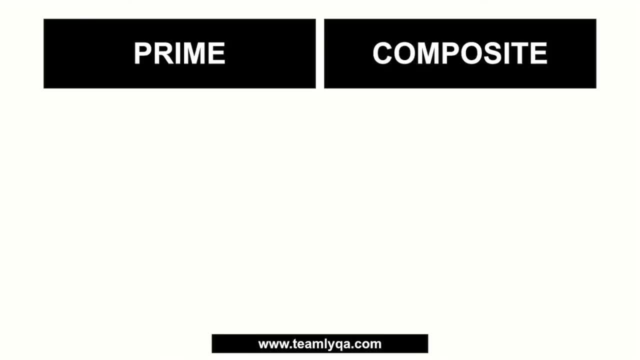 switch over to my PC. I'll see you in a bit. Alright, this is our lesson on prime and composite numbers. So first things first, we're going to define each one: The prime number and composite number. this is the quality of certain numbers And its definition is that the prime is a number. 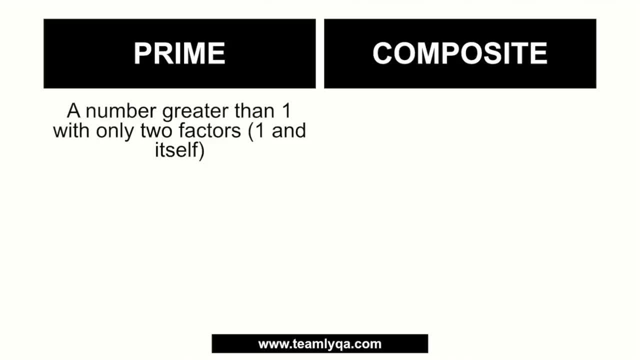 greater than one, with only two factors. Now, if you got a little bit confused with the term factor, this is the number that you can divide by. Okay, so it means that if a number is prime, it's a number that is greater than one, that its factors are only one and its own. We have 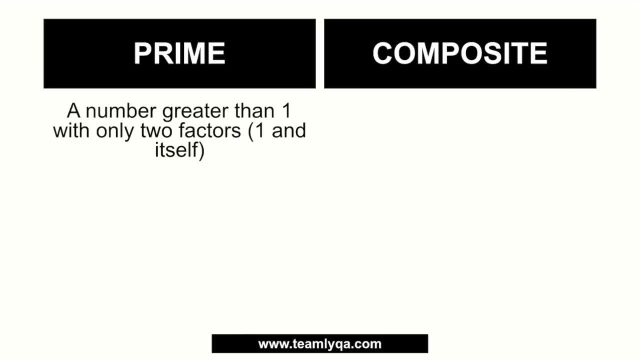 the identity property that is called multiplication, which is actually what this also implies, Because the identity property means that if you multiply any number by one, what will come out is its own, its own identity Number, same number will come out, And it means that the prime number is just its two factors. 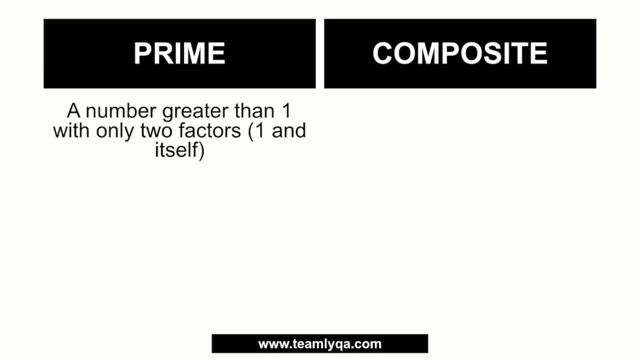 the one and its own, There's no other. Okay, and again, if you haven't watched my discussion on properties of addition and multiplication and you get a little bit confused with the identity- associative, commutative and distributive- I'll just link it here at the top so you can catch up. 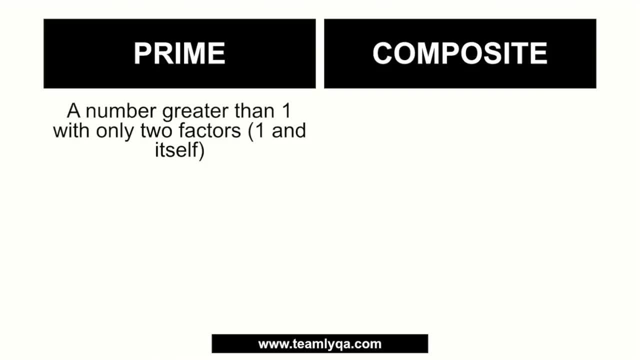 Okay, now we will play with examples later, which will help you remember this better. The composite number: it's different because it's a number with more than two factors. So it's greater than one, definitely, but its factors are greater than two. It means that 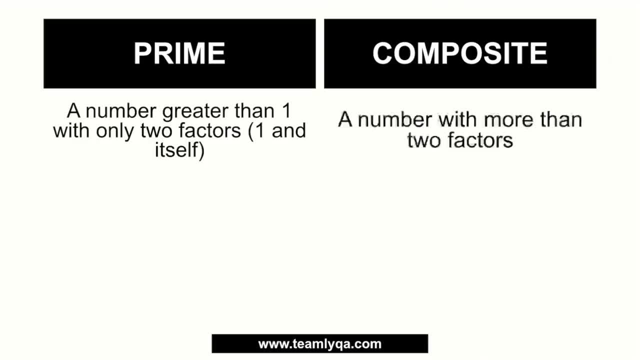 apart from one and its own, it can also be divided by two. it can also be divided by three, any other number besides one in itself. So let's take these two numbers as examples. Let's start with three. Let's list first its factors. So three. 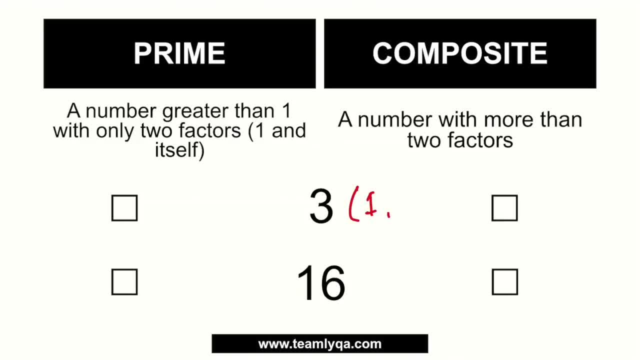 you can divide it by one. It will come out that three divided by one is three. But if you look at it, there's nothing that can be done. Okay, it can't be divided by two anymore, because it will come out as a decimal. 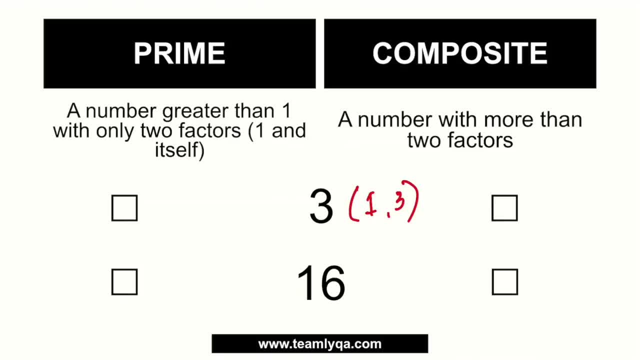 And there's no other number that's smaller than it. So it means that its factors are just one and three. So because it only has two factors, it means that it's a prime number. The sixteen is different because you can divide the sixteen by one, You can also divide it by two. 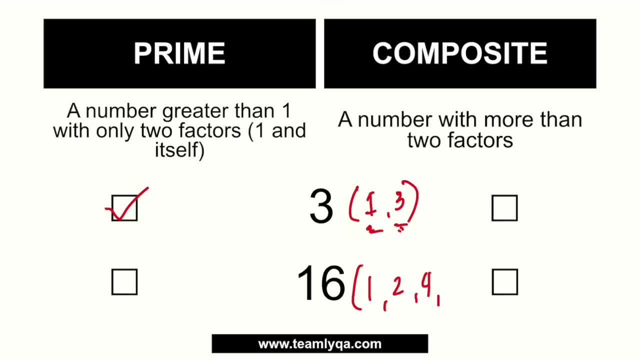 It can also be divided by four because it has two. it can also be guided by the eighth. It can also be by sixteen. Okay, so we have five factors here revolving mount. now, if someone is asking you sort of like Coach, how did you find out that it's divisible? 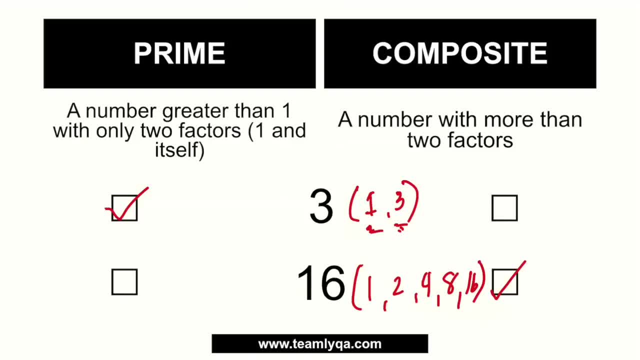 there are actually techniques on that And we're going to go through that a little bit later, but it's important for you to know that all the scores are a property of one person. The key point is: in order to win, you have to study the numbers. There are actually techniques on that And we're going to go through that a little bit later. 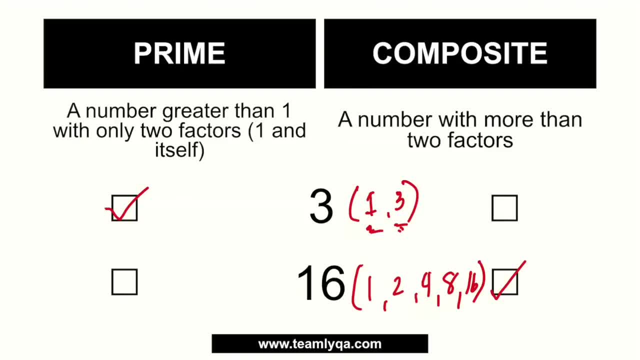 Pero ang importante dyan na skill is yung factoring. okay, Now a quick little side note. if you notice ang 16 ay even number, Any number na higit sa number 2 na even is automatically a composite number. 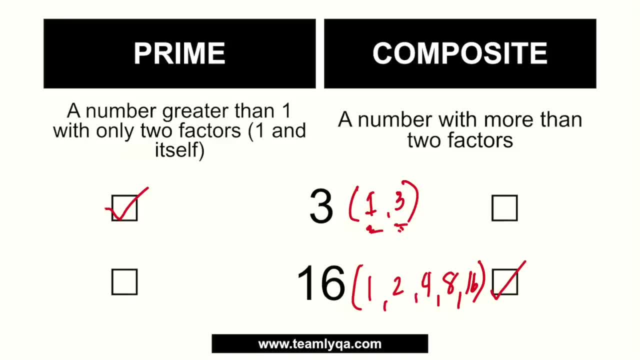 Bakit? Kasi lahat ng even numbers pwede mo sila i-divide sa 2. Yung 2 lang ang mananatiling prime, kasi ang 2, ang pwede mo lang na factor niya ay 1 at 2.. 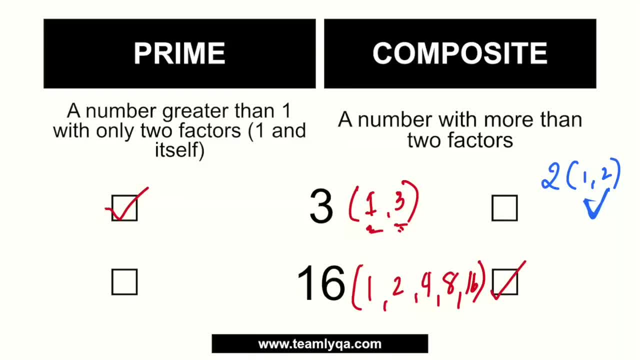 Wala nang iba. So ibig sabihin, dahil dalawa lang din siya, 1 in itself it still is a prime number, Pero pagpalo mo ng 4, okay, lahat yan composite na. 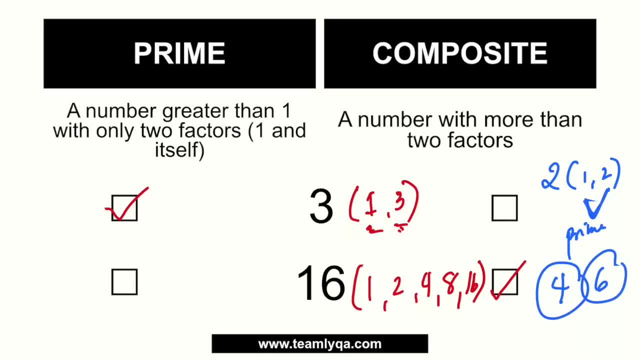 So 4,, 6,, 8,, 10, and so on and so forth. any even number greater than 2 becomes a composite number. Okay Kasi, automatic divisible siya sa 2.. Now what about 0 and 1?? 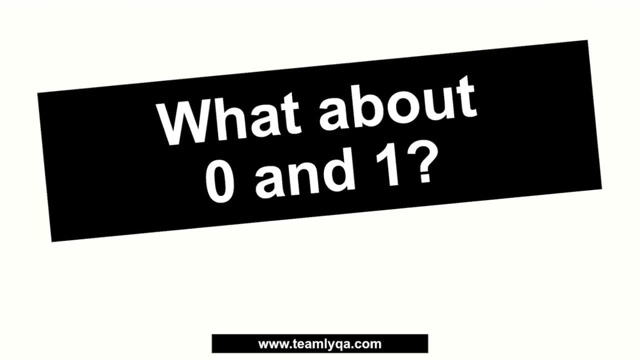 Ang 0 and 1 is considered as neither prime nor composite numbers. okay, Kasi mas complicated na lang yung sitwasyon nila. We're not going to dive deeper into this. You just need to remember that Again, kapag 0 and 1, they are neither prime nor composite. 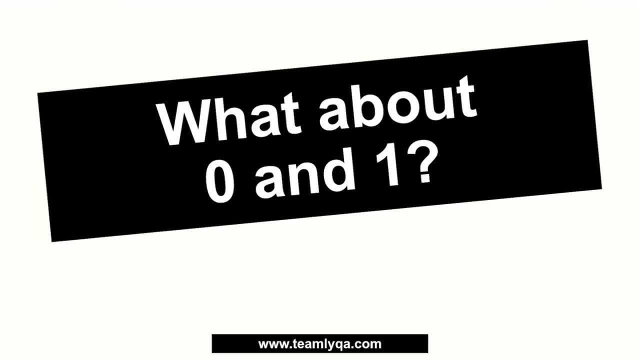 So, kung tatanungin kayo, ililist nyo kung ano-ano yung mga prime numbers, you don't start with 1 necessarily, You can start with 2 instead. Okay, Now meron na akong mga videos on factoring. 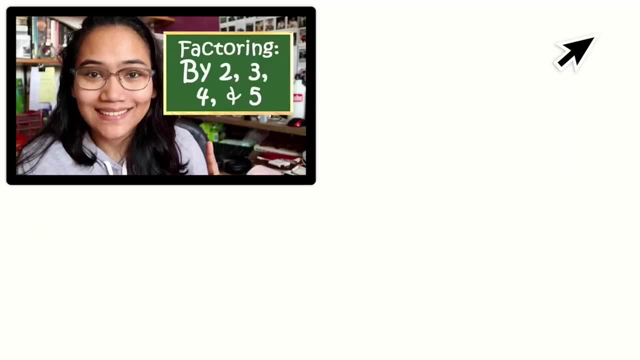 Meron ako on factoring numbers by 2,, 3,, 4, and 5.. Tinuro ko yung mga tips para mas mabilis nyo, Meron na siyang makuha. Meron na rin tayo yung 6,, 7,, 8, and 9.. 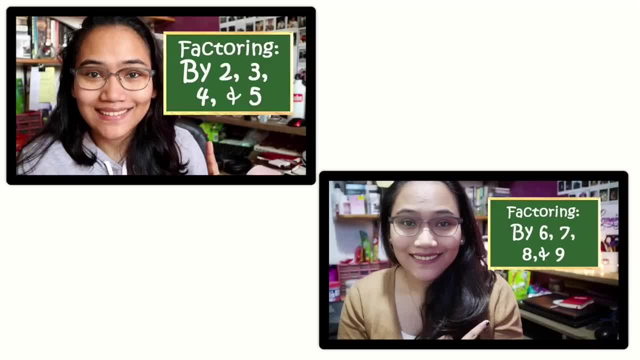 Ito yung pinaka-building blocks dito, Kasi ang pinaka-basic na gagawin ninyo to figure out whether a number is prime or composite is basically ask yourself, ira-run down yung lahat ng numbers na mas maliit sa kanya. 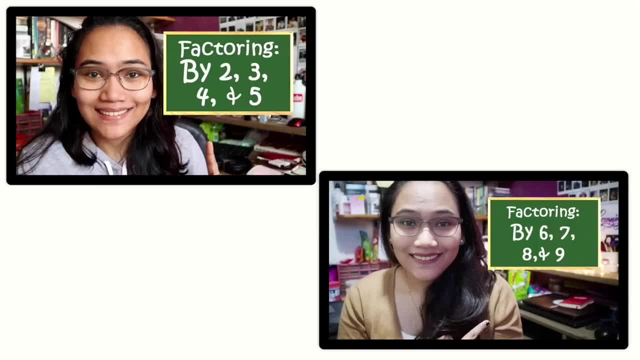 sino dun sa mga numbers na yun ang pwede mo i-divide sa kanya. At kung hindi nyo alam yung mga speed tips na ito, you may have to manually divide every number that you encounter. So imagine kung napakalaki yung number niya. 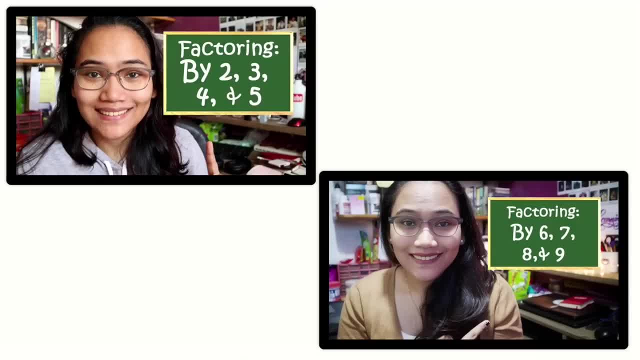 mahirap i-weed out kung ano yung prime or composite, Pero kung mamamaster nyo ito mas madali sa inyo. Mas paton, kung siya ba ay divisible sa any number other than 1 in itself. 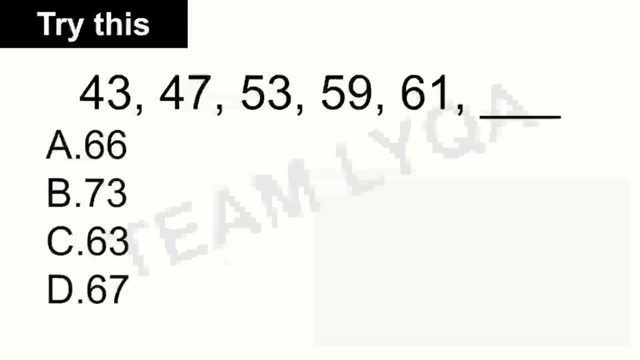 Now let's try this, for example. This is the type of question na nasa number series, pero it deals with prime and composite numbers. Bakit Kasi, if you solve this like a regular number series question, you would notice this. 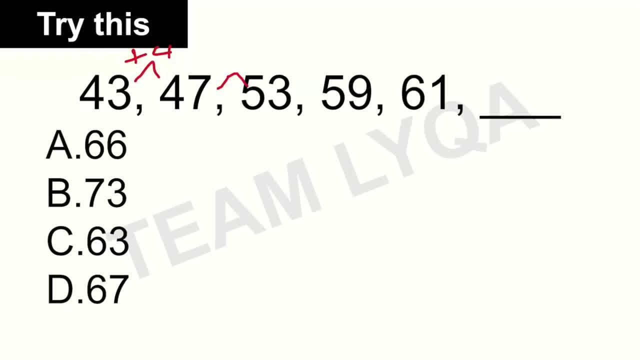 Ang relationship niya ay plus 4.. This- ang relationship niya ay plus 6,, which is different na sa plus 4.. And I also have a full length na discussion on this type of question na lagi lumalabas sa mga exams. 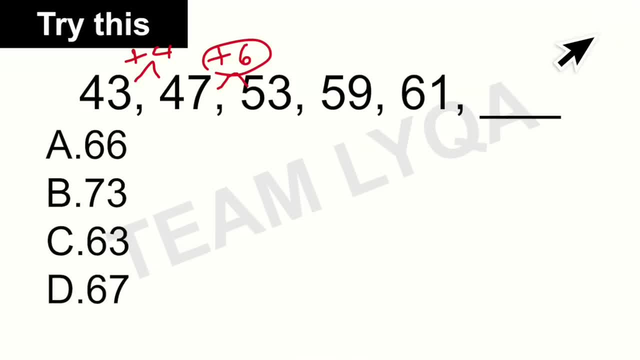 If you haven't seen that yet, ilalink ko na lang din dito sa taas ha, yung number series Marami nang natulungan yun, kahit yung mga ibang mag-e-exam ng NMAT. 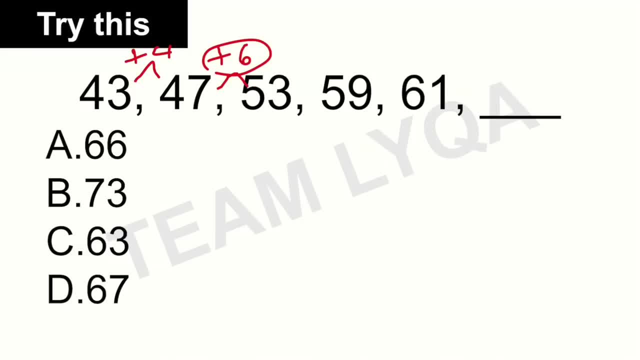 or Filsat or anything like that. So go ahead and watch that. Hindi yun necessarily ang goal ng lesson na ito. Ang goal natin dito is to figure out yung mga prime and composite numbers, Now yung 53 to 59, that is still plus 6.. 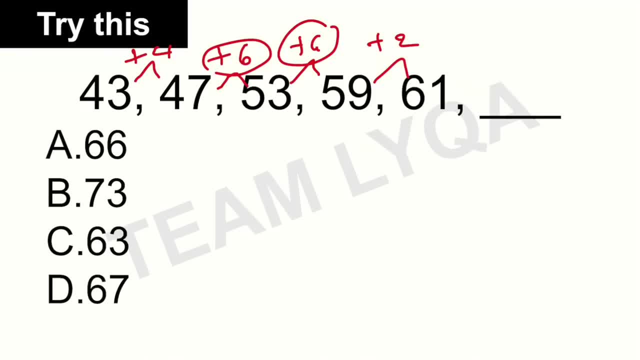 Ito ngayon ay plus 2.. If you notice, walang masyadong relationship itong mga ito, Kahit na mag-skip ako like this, this is plus 10.. Tapos yung 53 to 61, that is plus 9.. 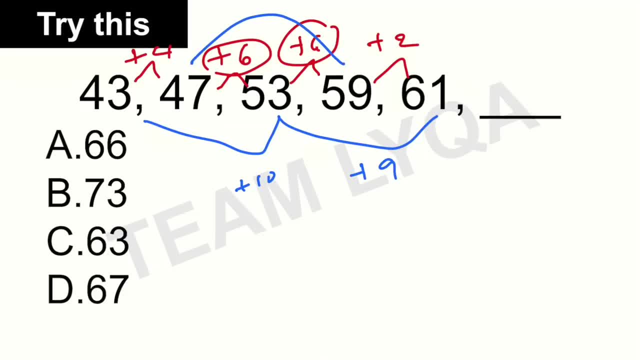 Walang relationship siya, Ito naman dito. wala rin siyang malinaw na relationship. This is basically plus 12.. So hindi mo makuha using yung common patterns that we have Now. ano ang magiging clue natin dyan? 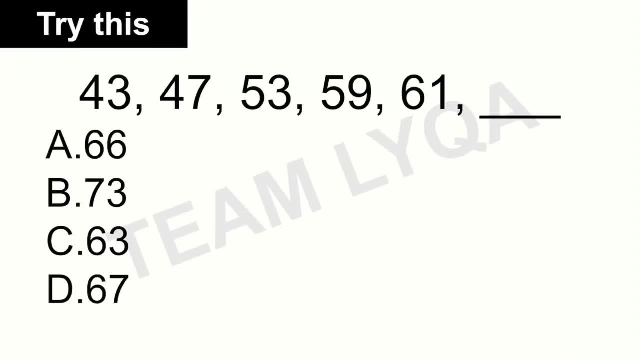 Now, if you notice, there is one thing in common with all of these numbers, which is all of them are prime numbers. Bakit Anong pwede mo i-divide sa 43?? It's only 1 and 43.. 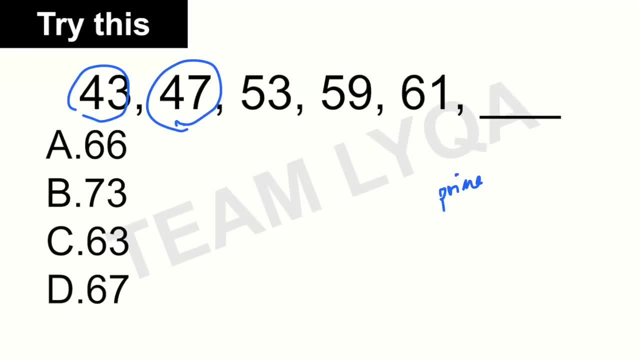 Ang 47,, ganun din 1 and 47, lang siya. 53 din hindi siya divisible sa any number besides 1 in itself. Ganun din ang 59 at 61.. So ibig sabihin nun: 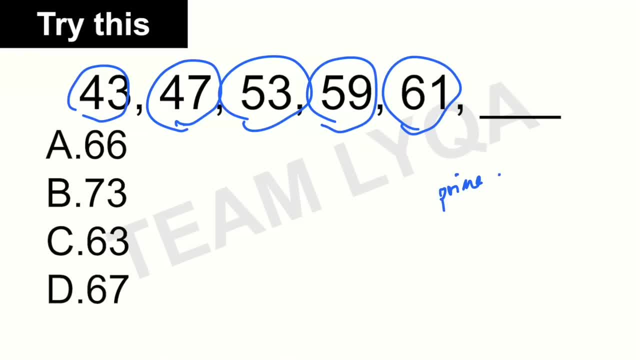 ang pattern nito is that ito ay list ng prime numbers, And all we need to do now would be to look at the options and see kung anong number na sinubukan. Ang susunod sa kanya na prime number din. 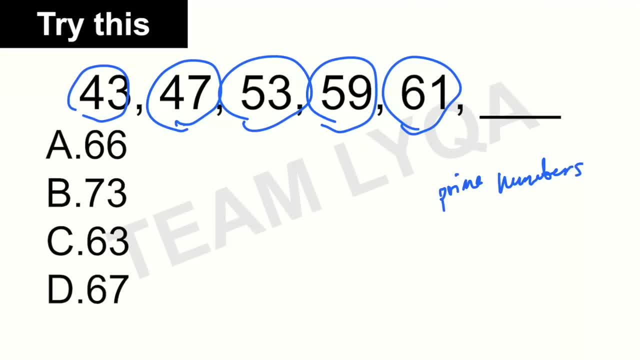 Now, ang style ko sa exams, when I encounter questions like this, is I start with yung pinaka maliit na number, Kasi 61 siya. So titinan ko anong pinaka maliit na number dito. 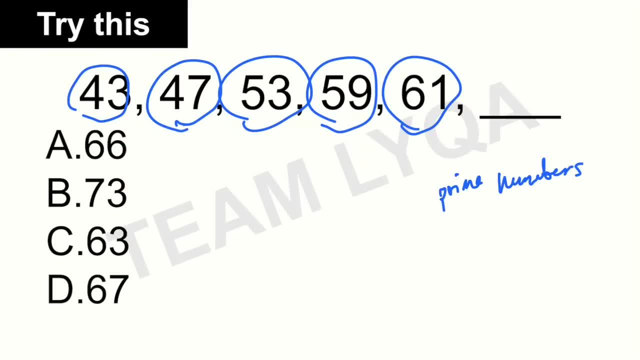 Ito is 63.. Ibig sabihin siya pinaka malapit sa 61.. I'll ask myself: ito ba ay prime or composite number. Now, off the bat, kita ko na pwede mo siyang i-divide. 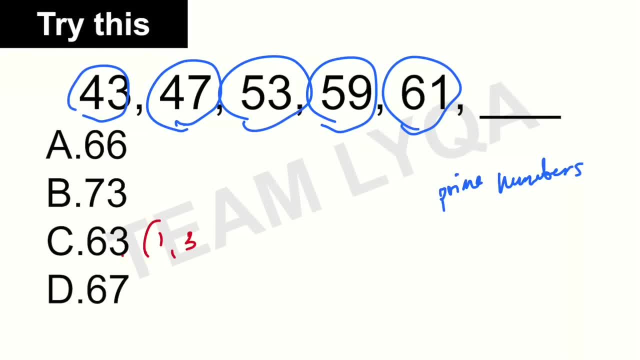 Maliban sa 1, pwede siya sa 3.. Okay, Kasi yung 6 and 3, ang rule natin sa factoring ng 3s is pag in-add mo yung kanyang digit. so 6 plus 3, that is 9.. 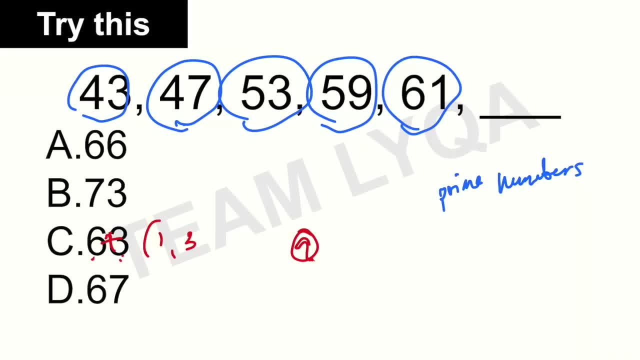 At kung divisible yan sa 3,, ibig sabihin divisible din yung big number ng 3.. So ibig sabihin: pwede siya sa 3.. So ibig sabihin: nun, hindi ito prime number. 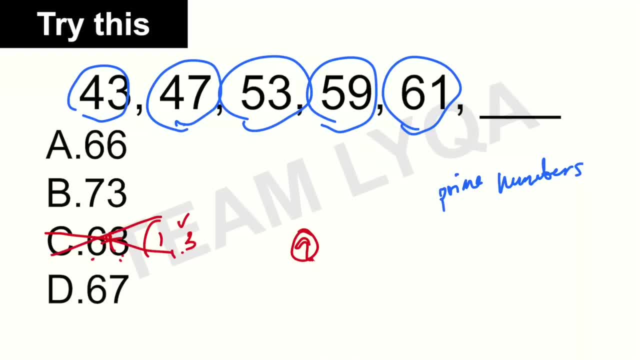 siya ay composite number. And again, kung naiwan kayo dun sa speed technique na yun, panoorin niyo muna yung video ko on factoring by 3 para makuha niyo yung technique. 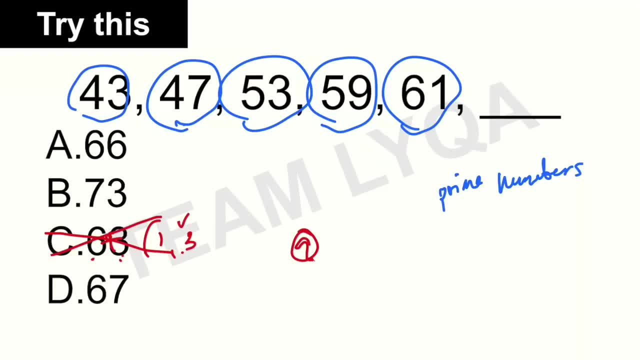 Now. so ibig sabihin ang 63 is out of the way. Hindi na siya pwedeng option. Tingnan natin yung 66.. Ang 66 is an even number. Okay, Kasi it ends with 6.. 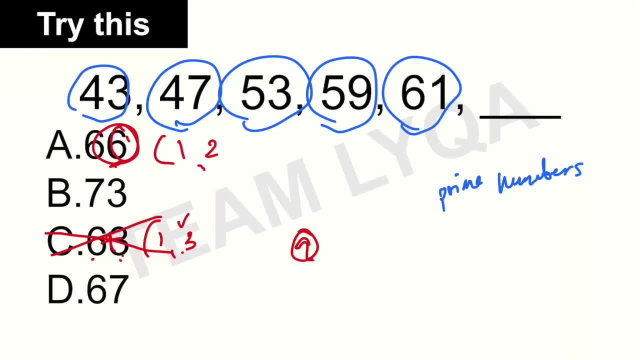 Ibig sabihin, pwede mo siya i-divide sa 2.. So maliban sa 1, meron ka na agad 2.. I will stop at that, Hindi ko na kailangan ilista lahat. 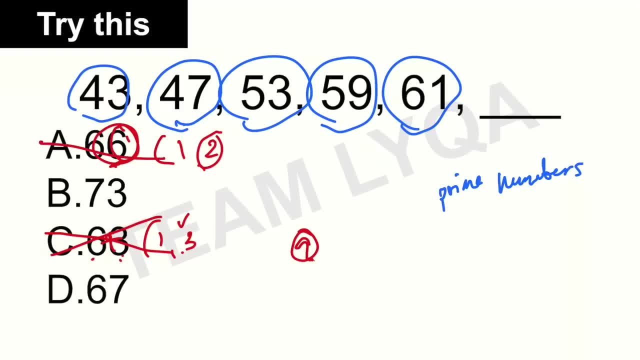 Kasi nakita ko may 2 na agad. Ibig sabihin ito ay composite number. Hindi na rin siya pwedeng sagot, So dito ako sa susunod, na sa 67.. Ang 67, hindi siya even. 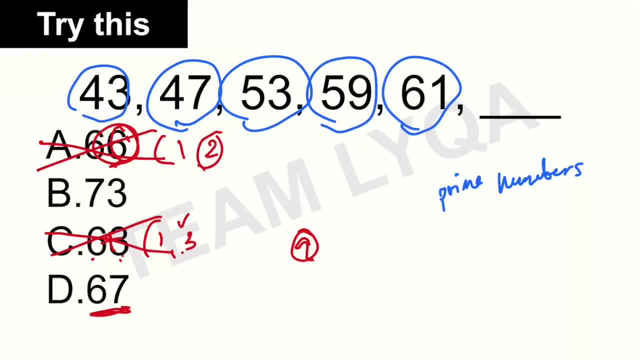 So hindi siya pwede sa 2.. Hindi na siya pwede sa 3.. At dahil hindi niya even, hindi siya pwede sa 4.. Hindi na siya pwede sa 6 or any other number. 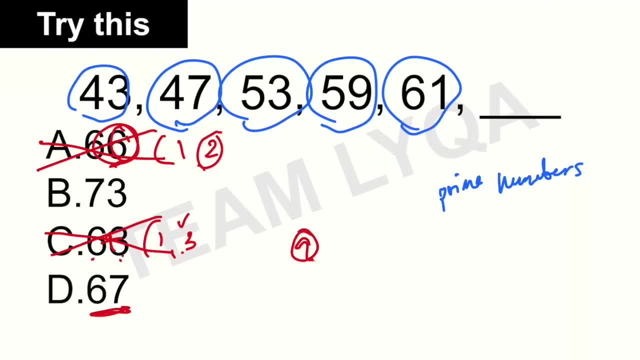 So ibig sabihin, dun ang 67 can now be an option. for me, Ang 67, now becomes a prime number. So kung prime number ang 67, at siya ang pinakamaliit na kasunod ng 61,, 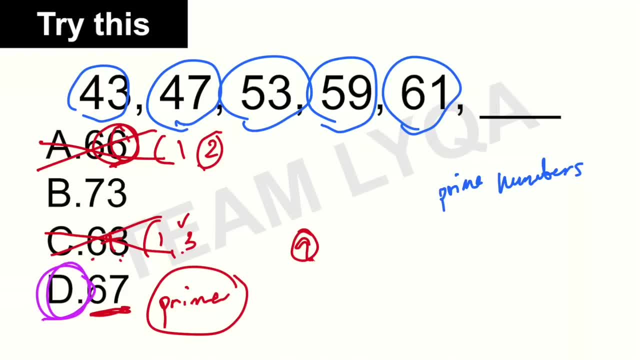 then ibig sabihin nun, ang answer ko now is 67.. Okay, So again it plays a huge part doon sa pagsusolving natin ng mga problems sa math. Kasi, kung hindi mo nga alam, 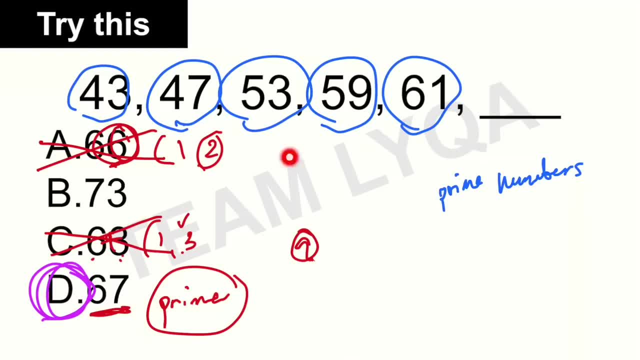 kung ano ibig sabihin ng prime number. you will have difficulty with this type of number series question, which I already encountered in other exams that I take. There are also word problems na sasabihin what is the sum of all prime numbers. 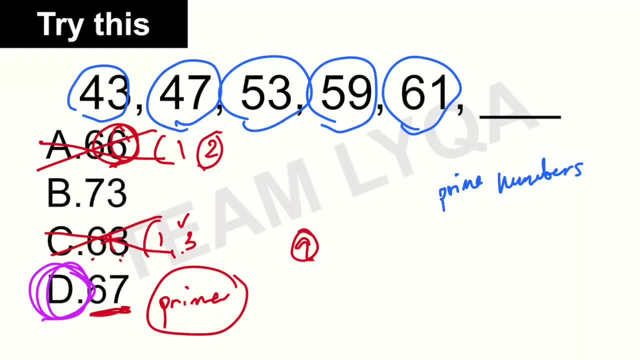 lower than 20. Something like that. So kung hindi mo alam kung ano yung prime, hindi mo maililista yung mga yun, hindi mo rin sinama-add. So very important for you to learn kung ano yung difference. 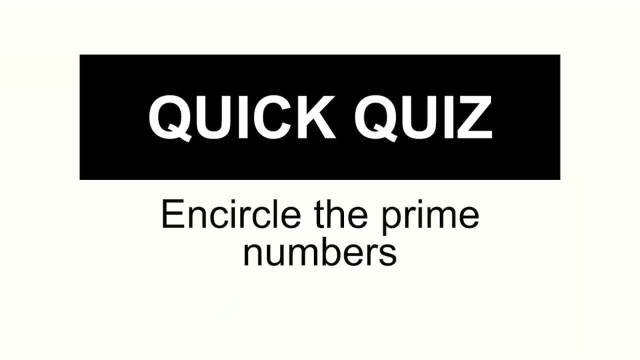 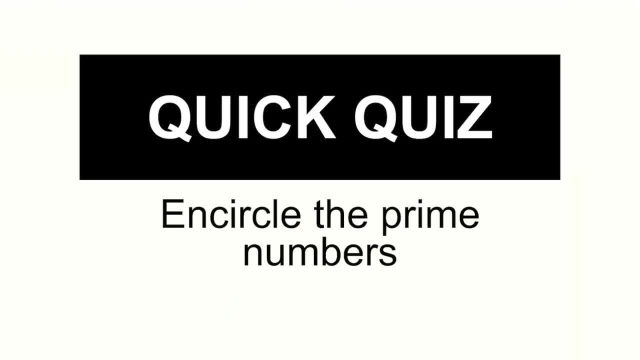 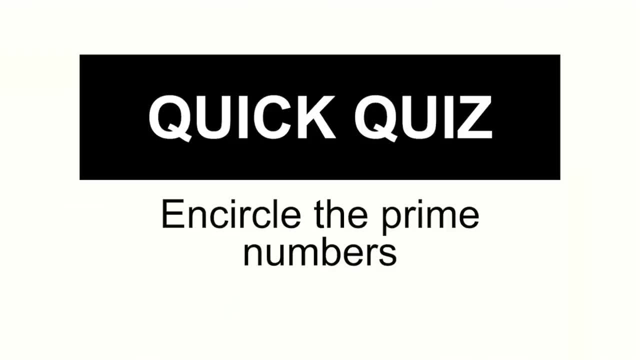 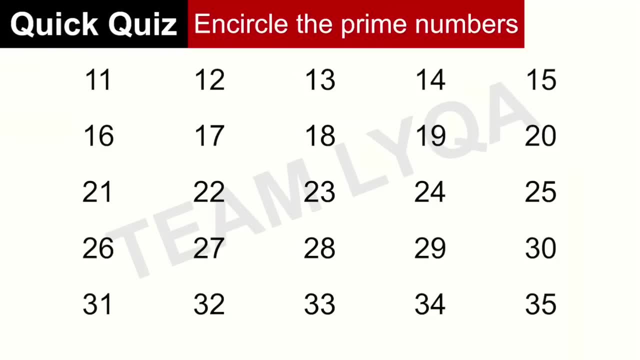 Balikan nyo na lang yung mga video lessons. na yun, mamaya, Okay, And if you're ready with your pen and paper, your timer starts now. arni ango, yco, yco, yco, yco, yco, yco. 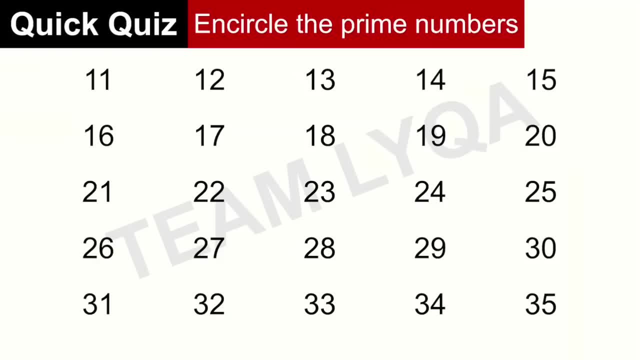 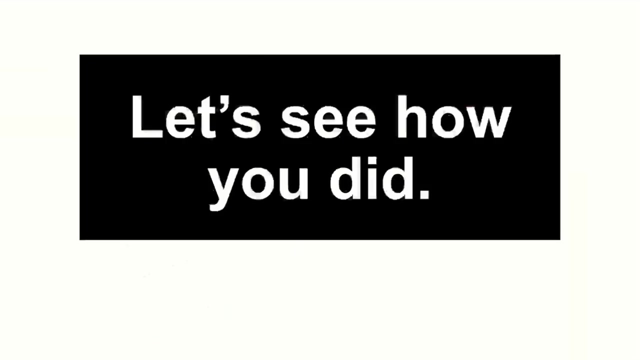 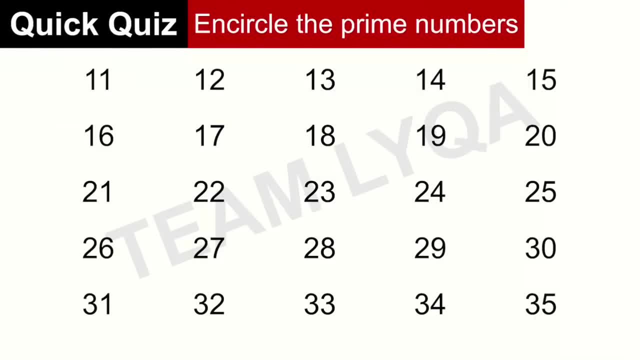 Now 11,. can I divide it by 2?? No, I can't divide it by 3.. No, I can't divide it by 3.. No, I can't divide it by 3.. Actually, you can divide it by 11,, but not 1 in itself. 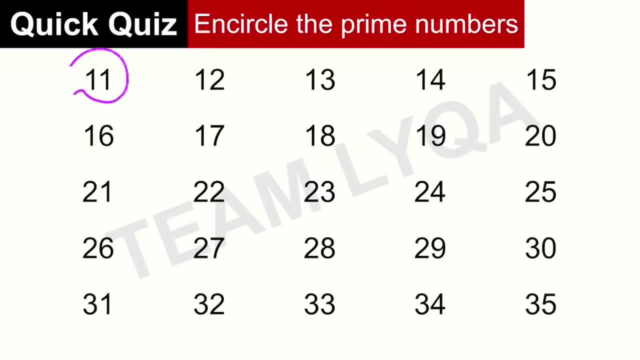 So it means that this is a prime number. So I'll round it. Okay, 12 is an even number, So even then it can't be a prime number, So it's not included. And again, like I said earlier, 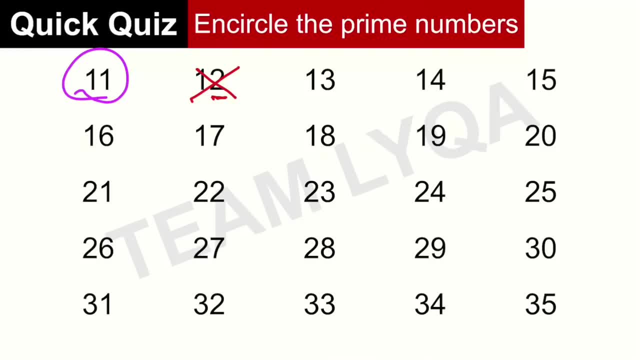 any number bigger than 2, an even number is not a prime number because it's divisible by 2.. I can rule out all even numbers. If you didn't do this earlier, at least now you know, just in case you encounter a question. 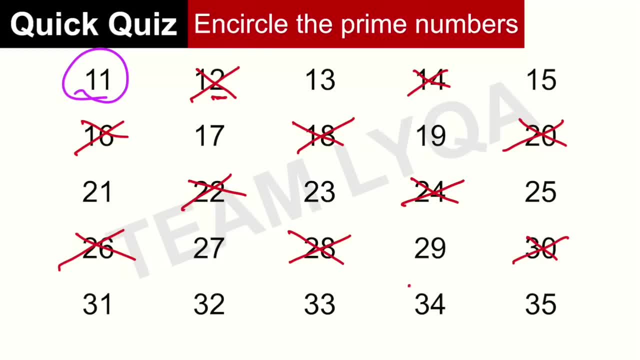 like this, or if you have the opportunity to showcase this. you know immediately, automatically it can't be an even number, But that doesn't mean that all odd numbers are prime numbers. All I need to do now is to assign them. 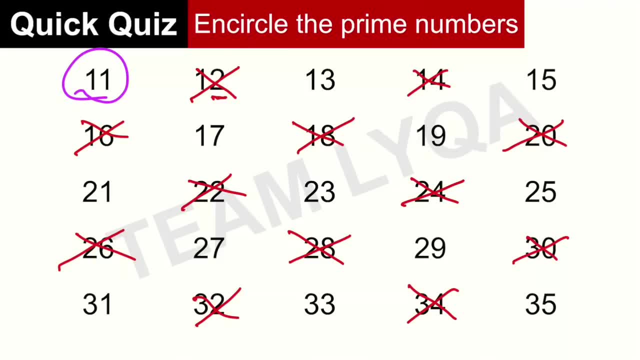 Now 13,. I can't divide it by any number other than 1 and 13.. So it means that it's a prime number, 15,. I can divide it by other than 1, it can be divided by 3.. 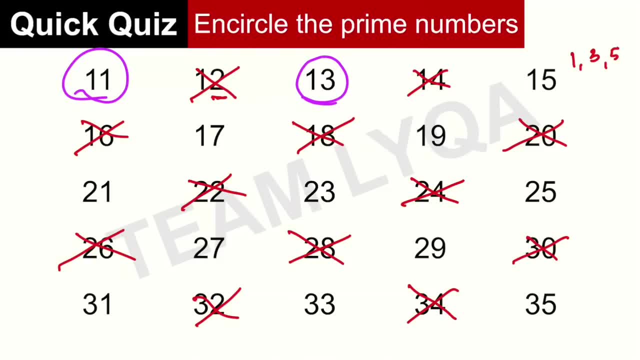 It can also be divided by 5. So it means that it's not a prime number, It's a composite number: 17,. well, 17,. I can't divide it by any number other than 1 and 17.. 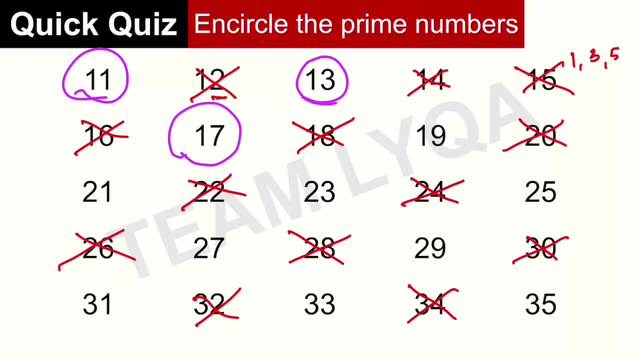 So it means that 17 is included, 19, it's the same. It's not divisible by 3, or any number smaller than 19, other than 1 and itself, So it means that it's also a prime number. 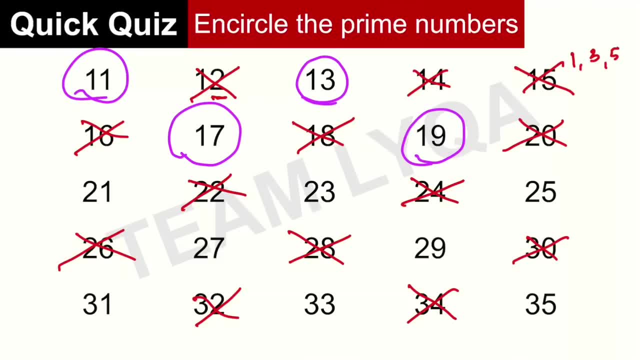 21,. it's not even yes, But actually I can divide it by other than 1, it can be divided by 3. The 7 will come out, So it means that it's definitely not a prime number. 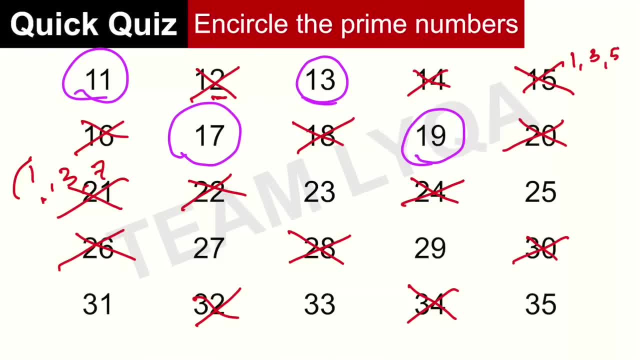 I can now remove it. 23,. it's not even, but it can't be divided by 3, it can't be divided by 4,, 5,, 7, there's no other number that you can divide it by. 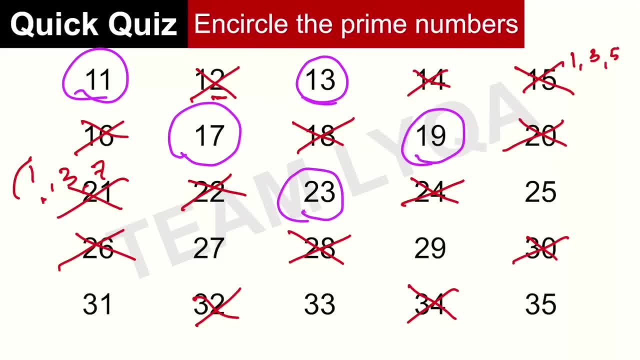 So it means that it's a prime number, 25,. well, it can't be divided by 2, but it can be divided by 5, because 1, 5 times 5 is 25.. So it means that: 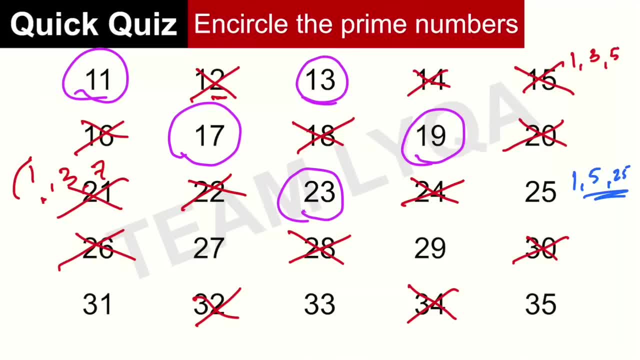 I can divide it by more than 25 and 1.. It's more than 2 factors. It means that it's a composite number. It can't be answered 27,. it can be divided by 9 times 3.. 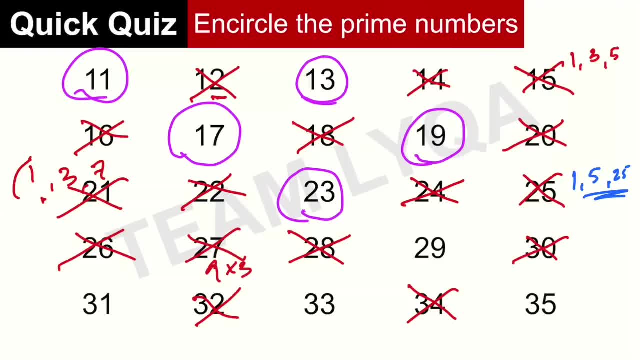 So it means that it can't be divided by 9, because it's not 1 and itself 29,. hmm, it can't be divided by 3.. It can't be divided by 2.. It can't be divided by 6.. 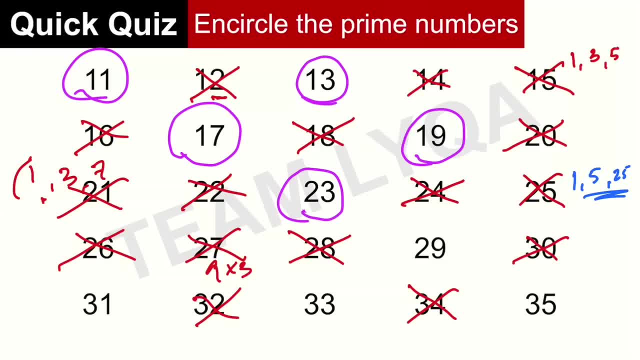 It can't be divided by 7.. It can't be divided by 9. So there's no other number. So it means that it's a prime number 31,. it's the same, It's a big number. 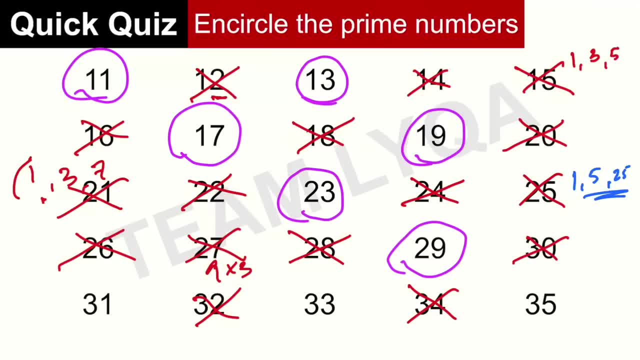 but it can't be divided by 3,, it can't be divided by 6,, it can't be divided by 7 or 9,, even 11.. So it means that it can't be divided by anything other than 1 and itself. 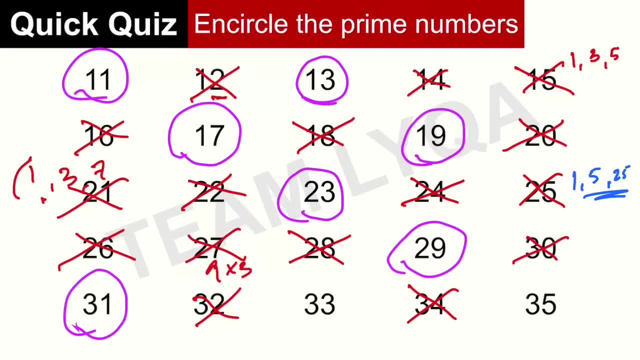 That makes this a prime number. 33,. okay, it can be divided by 3,. it can be divided by 11.. So it means that there is more than 1, and itself It means that it's a composite. 35,. I can divide it by 5 and 7.. 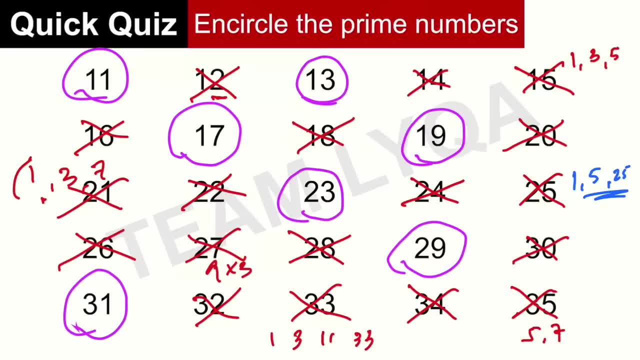 So it means that it's also a composite number. So what we have here would be 11,, 13,, 17,, 19,, 23,, 29, and 31.. Now, I hope you got all of those correctly. 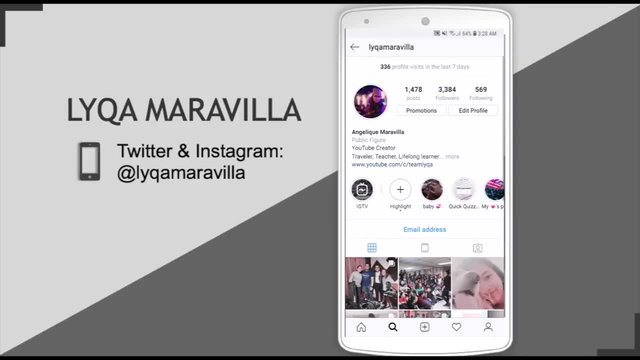 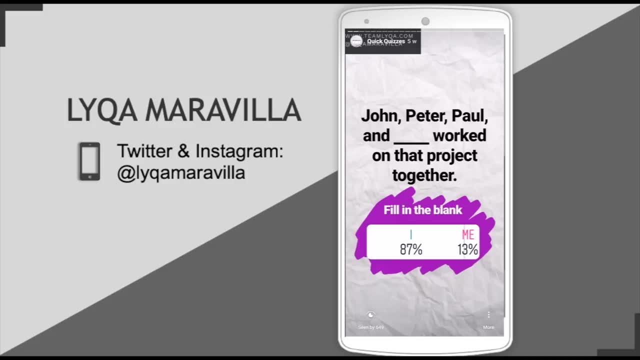 If you didn't, that's okay. I'll be posting more questions on my Instagram account. So if you don't follow me yet, follow me at Laika Maravilla for more quick quiz questions And, as always, I'll check the questions that I post on my Instagram story. 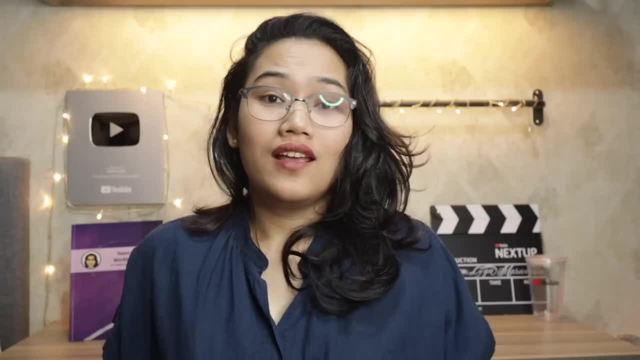 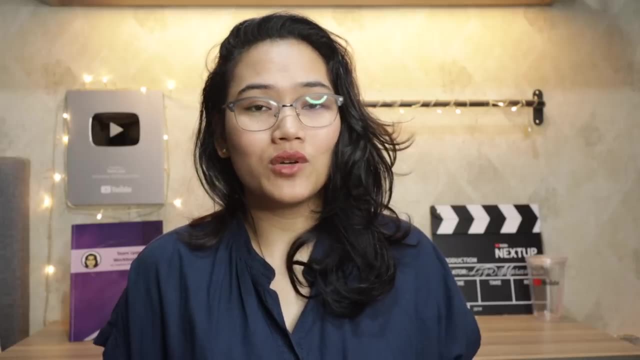 Your name should be one of the correct ones. Okay, Alright, I hope you learned something today. If you didn't click thumbs up, Make sure to share this video with your friends. That way, we can help each other more. And, as always, if you want to reach out to me directly, 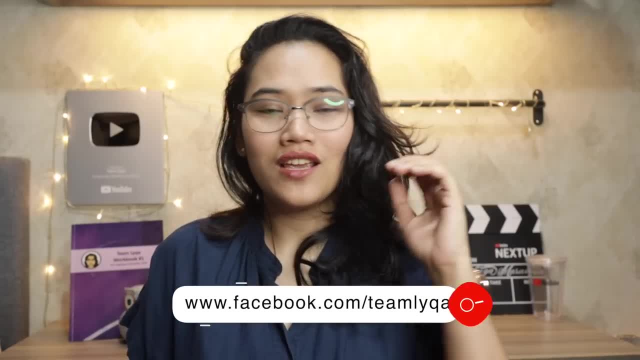 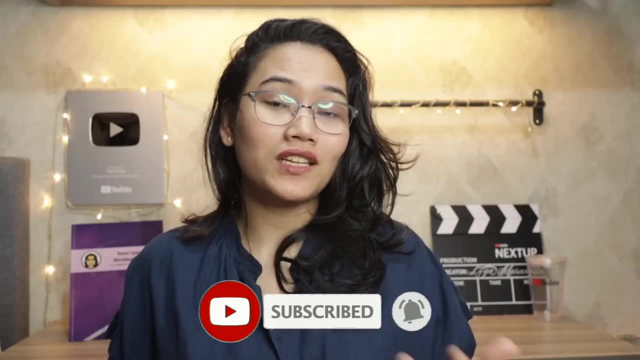 get the reviewers join the online or live review events, or just catch me on my next speaking engagement. you can follow me at wwwfacebookcom: slash team Laika Subscribe if you haven't yet Hit that bell icon, so you don't miss the upcoming lessons. 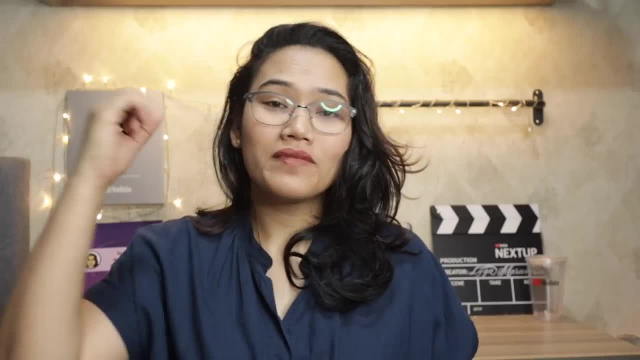 We have more coming up. I'll see you in the next video. I'll see you in the next video And bye for now.